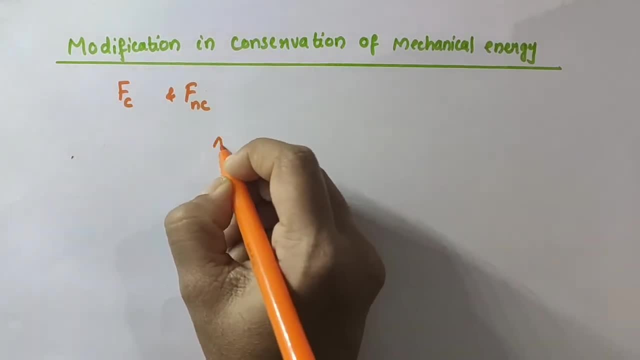 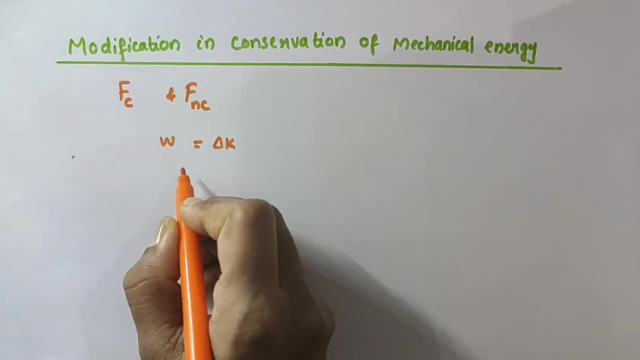 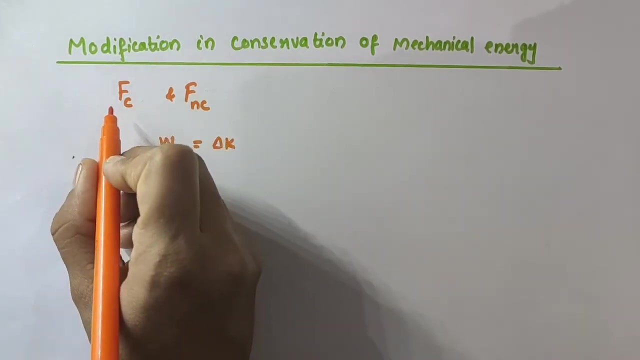 By the work energy theorem, the change in kinetic energy of a particle. change in kinetic energy of a particle is equal to the work done on it by the net force. So here we have a conservative force and a non-conservative force. So the work done will be the work done by the conservative force plus work done by the non-conservative force. 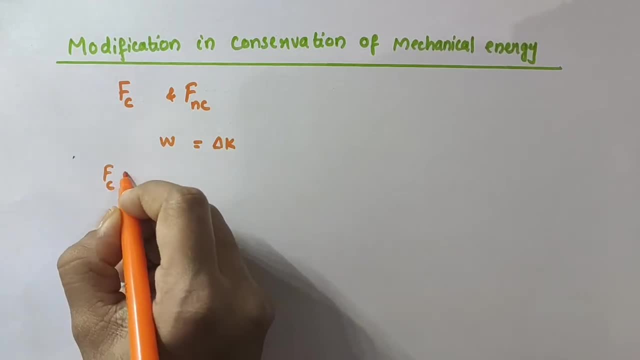 So we can write that work done as work done by the conservative force can be written as Fc. Okay, we are just considering the one-dimensional case and so force into displacement. We are using the formula work done is equal to force into displacement. 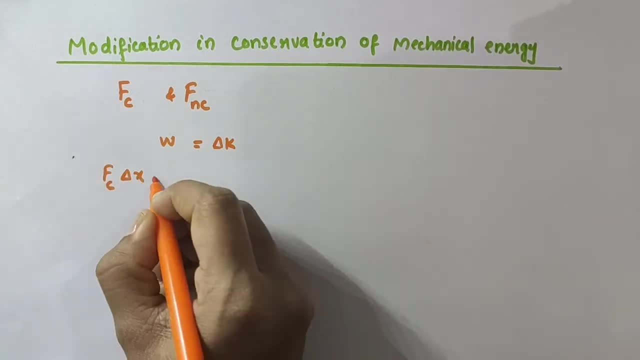 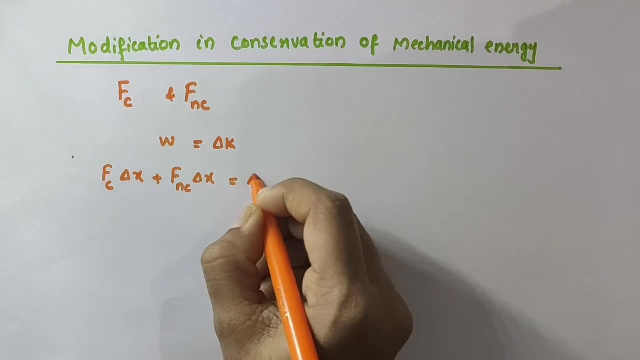 Okay, we are considering the one-dimensional case. So Fc into delta x plus work done by the non-conservative force, that is, Fnc into delta x, where delta x is the displacement. Okay, this is equal to delta k work done. that is equal to work done by the conservative force plus work done by the non-conservative force. 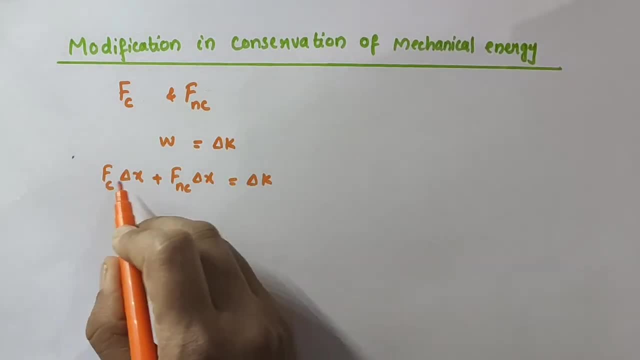 We are considering the one-dimensional case, So work done can be written as 4k. Okay, So this is the work done by the conservative force. then it is given as Fc into delta x. plus Fc wanna be equal to minus delta k. 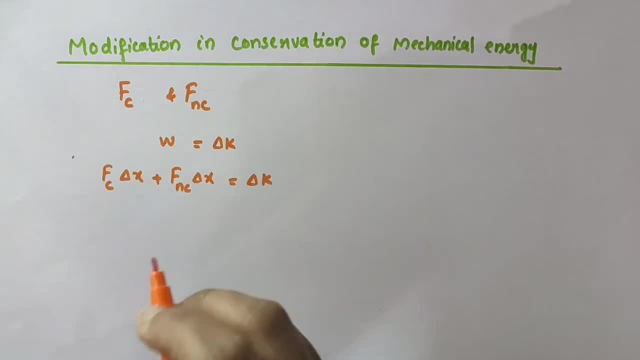 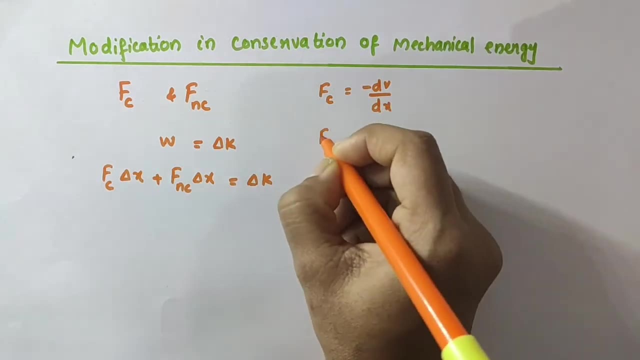 So we want it to be a nice ah, and if the event work done earlier this time, like this I will give you here, is a��sm works done by lazy function, Okay, so now let's try the, so we can write this work done. 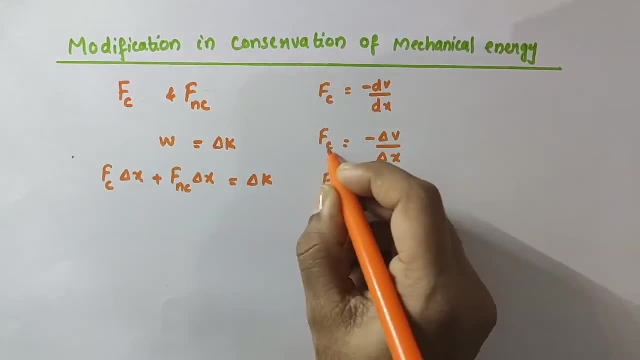 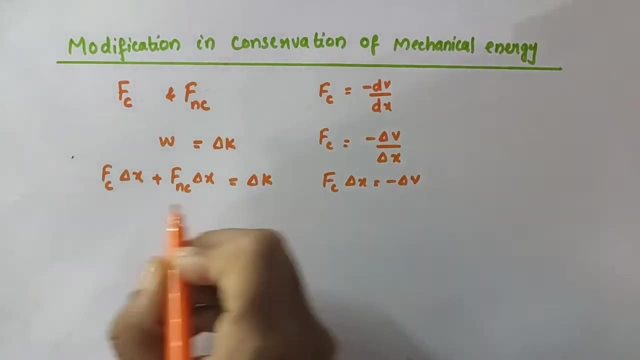 So for this, If one-dimensional case, we want it to be minus delta 2.. Okay, what does this tark me into? how this works? So it looks like h. What this h looks like. hey, Okay, fc into delta x as minus delta v here in this equation. so this equation becomes minus delta v. 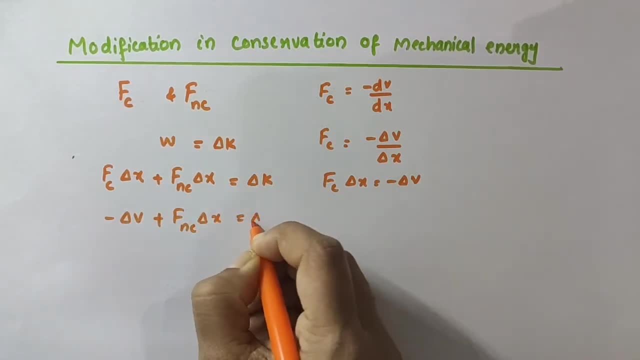 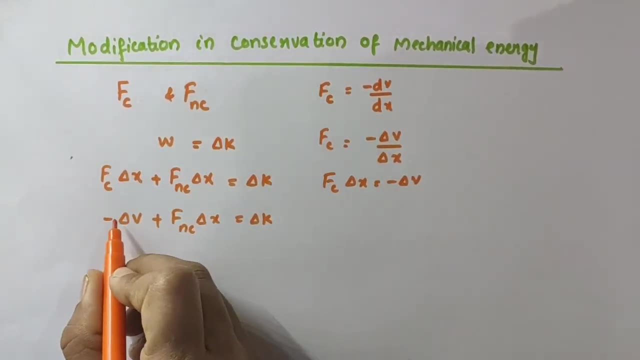 plus fnc into delta x is equal to delta k. all right, next what i'm doing is i'm just taking- uh, i mean i'm just taking this minus delta v to this set so that becomes plus delta v. so here we have: fnc into delta x is equal to delta k is already here. i'm taking this minus delta v to. 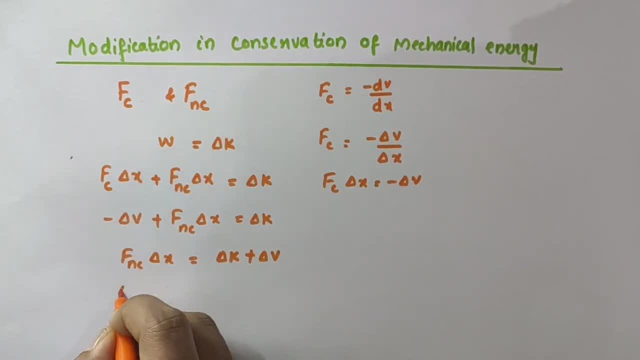 this set so that becomes plus delta v. all right, so here we are getting an equation: change in kinetic energy plus change in potential energy is equal to the work done by the non-conservative force, that is, fnc, into delta x. now we can write like this: now, delta of k plus v is equal to fnc. 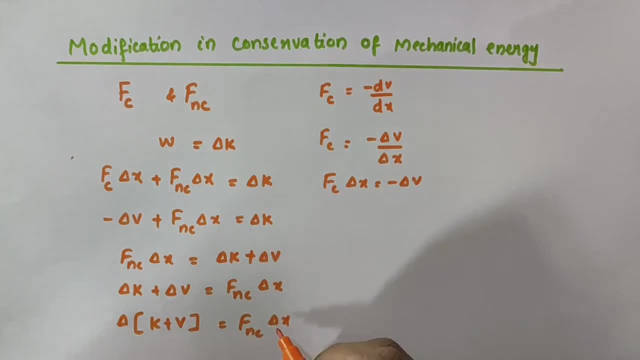 into, sorry, fnc, into delta x. okay, so change in: uh, kinetic energy plus potential energy. what is this? kinetic energy plus potential energy? that is the total mechanical energy, you know. so i'm representing it by e. all right, so we can write: change in total mechanic. i'm sorry, change in the total mechanical. 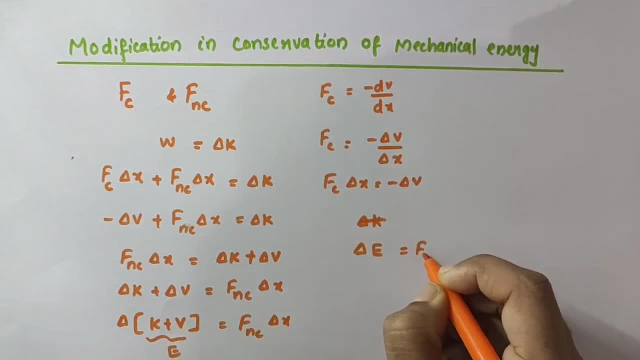 energy. e is equal to fnc into delta x. so change in total mechanical energy means final energy minus initial energy, initial total mechanical energy. okay, this is equal to fnc into delta x. that is actually the work done by the non-conservative force. that is why wnc okay. 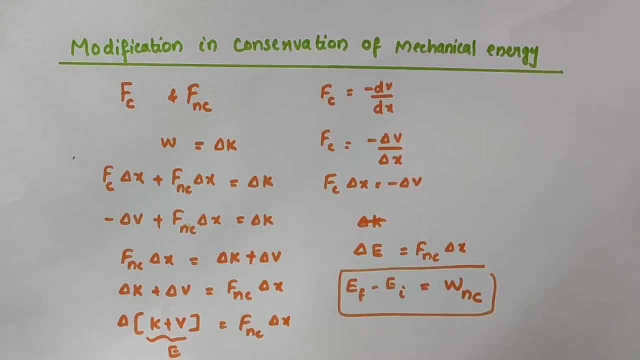 work done by the non-conservative force. now you see here the total change in- i mean the change in total mechanical energy- is actually equal to the work done by the non-conservative forces over the path. that is see, the change in total mechanical energy is not zero here, when we consider the conservation of mechanical energy. 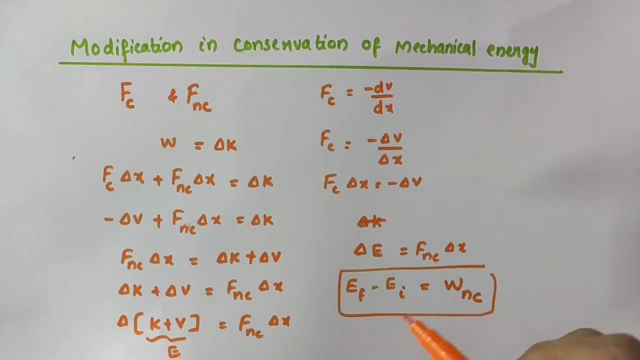 if the force is doing work on it, i mean the on that system is conservative, then we would get the change in total mechanical energy as zero. okay, because total mechanical energy is conserved in that case. so change will be equal to zero. but here the change in total mechanical energy is not zero. that means here in this case, that is, if there 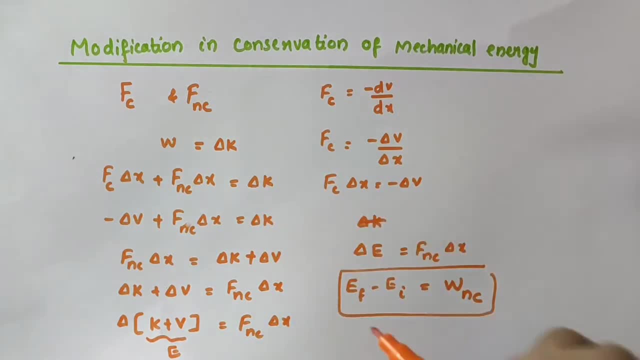 is a non-conservative force acting on the system, acting on a body, then the- i mean the total mechanical energy is not conserved. that is, there will be some losses in total mechanical energy which gets dissipated as sound energy, heat energy etc. so the total change, i mean the change in total. 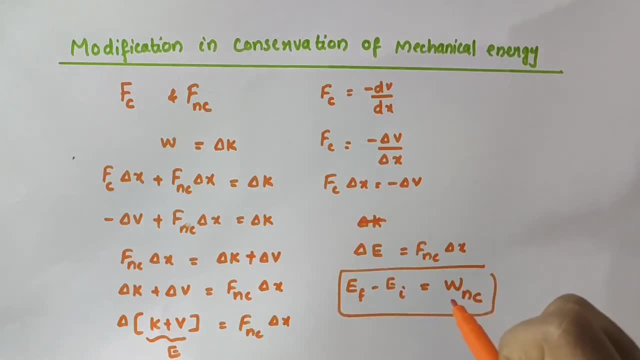 mechanical energy in that case will be equal to what the work done by the non-conservative forces over the path. actually the work done by the non-conservative- i mean a non-conservative force, no, a non-conservative force, that is actually a path dependent force. it depends on the particular. 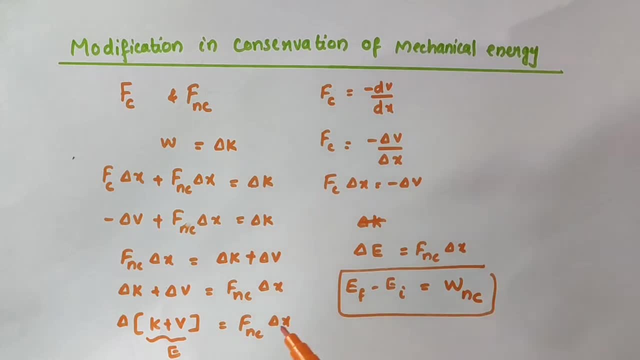 path from i to f. i is the initial position, f is the final position. all right, so in this video we have discussed about a very simple topic, a small topic, that is, modification in conservation of mechanical energy formula. actually, if the forces acting on the body is only a conservative, 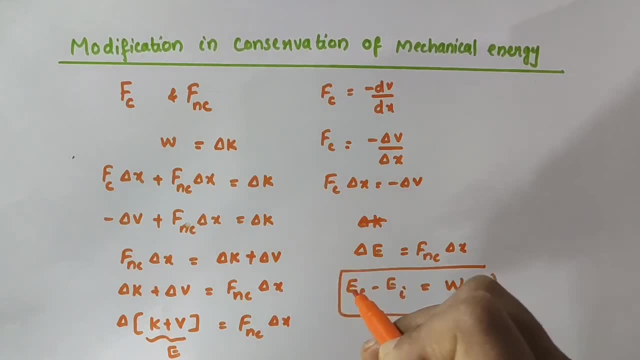 force, then the total change in mechanical energy- this ef minus ei is equal to that- will be equal to zero. okay, because total mechanical energy is conserved if the forces doing work on it are conservative. but here, if there is a non-conservative force acting on that body, then the total 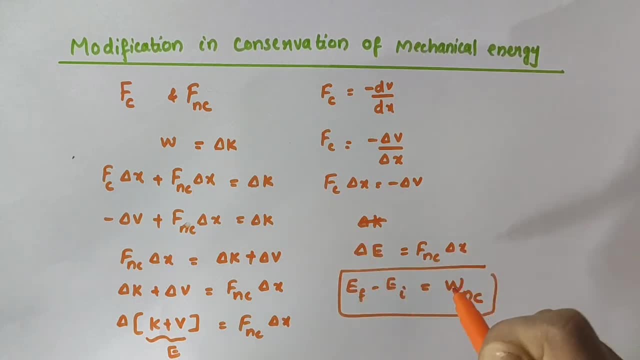 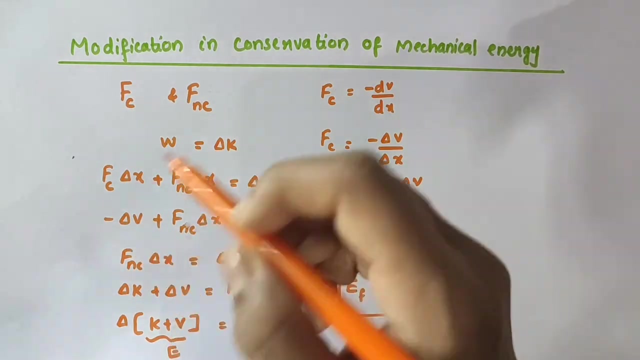 mechanical energy. change in total mechanical energy. that will not be equal to zero. instead that will be equal to the work done by the non-conservative force. that means the change in total mechanical energy is not zero. if a conservative forces, they are acting on that body, so there will be some losses in that total mechanical energy that gets. 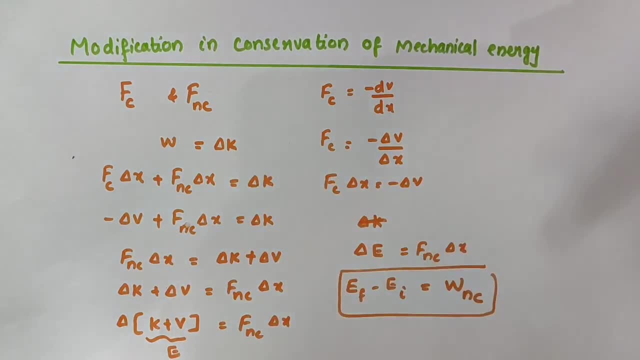 dissipated as sound energy, heat energy, etc. i hope you understood this, thank you. 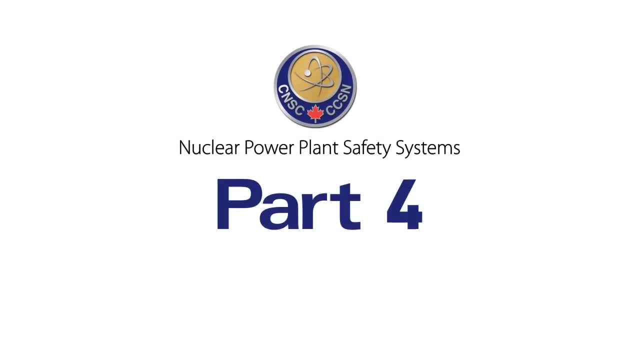 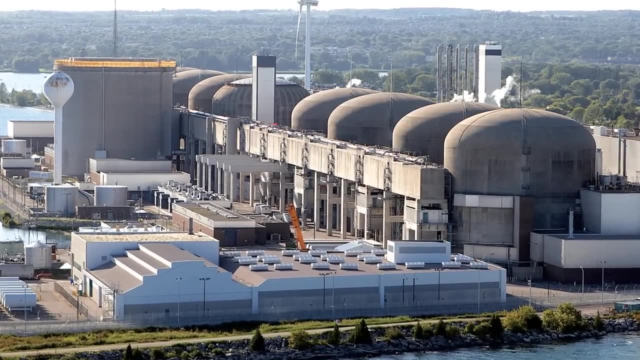 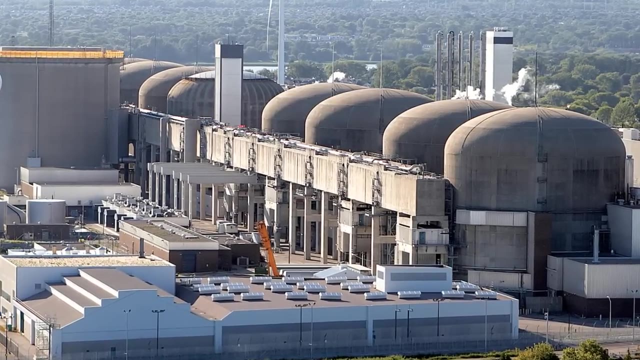 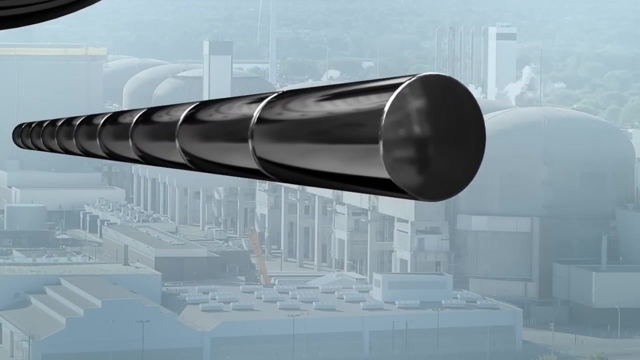 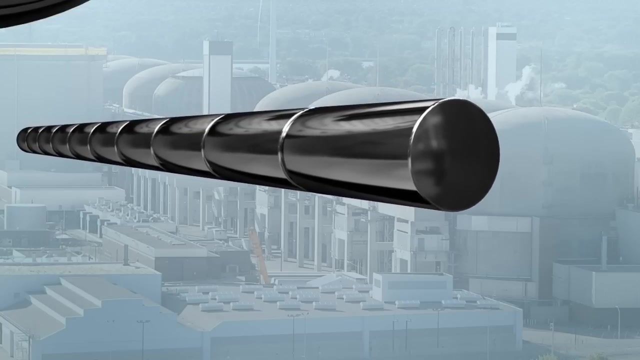 Now let's look at the third basic function: containing radiation. Nuclear reactors are built with multiple barriers to safely contain radiation. At the heart of all CANDU reactors are hardened ceramic pellets made of natural uranium. These pellets contain the radiation. They form the first layer of containment. The pellets are contained in rods which form 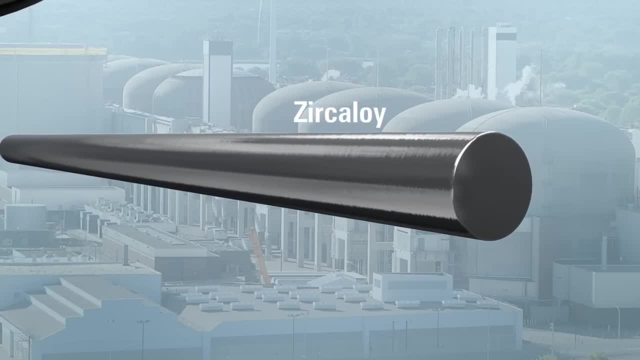 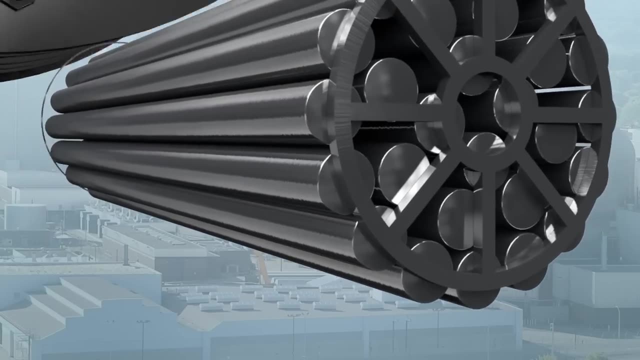 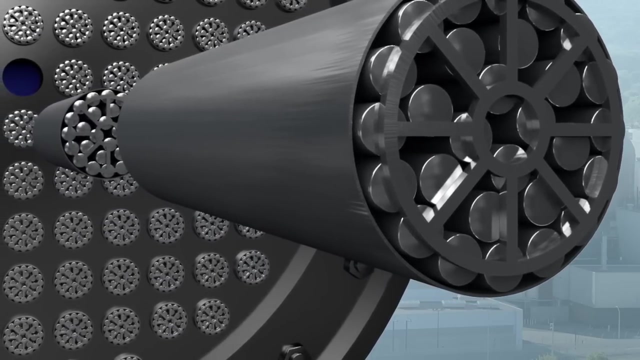 the second layer of containment. CANDU fuel rods are made of zerk alloy, a metal alloy extremely resistant to heat and corrosion. The rods are then loaded into pressure tubes, which are part of the heat transport system. This is the third layer of containment. 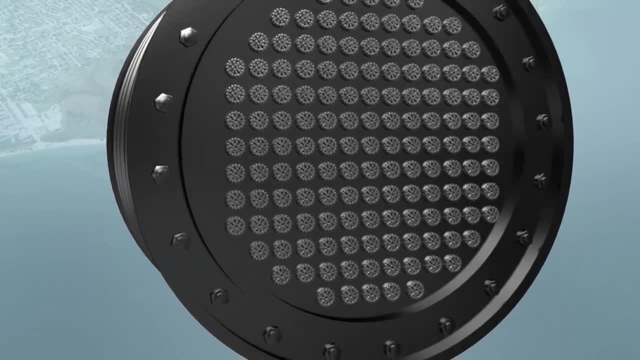 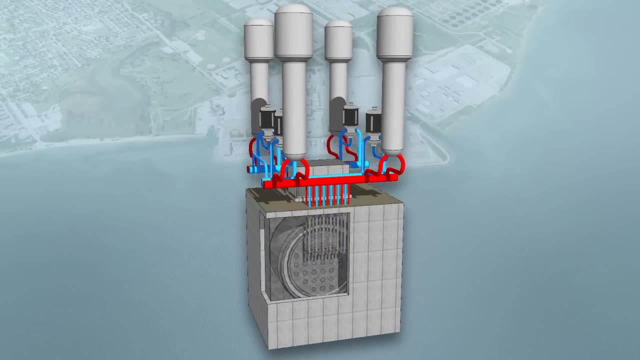 The pressure tubes are contained inside a metal tank called the condenser. The condenser is a solid-state reactor that is located in a hole in the middle of the reactor. The condenser is a solid-state reactor, or calandria, which itself is contained inside a thick vault. 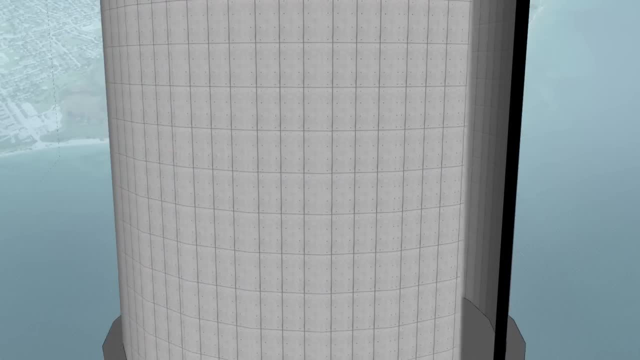 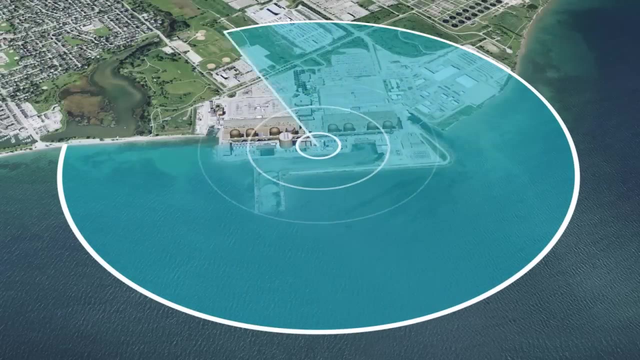 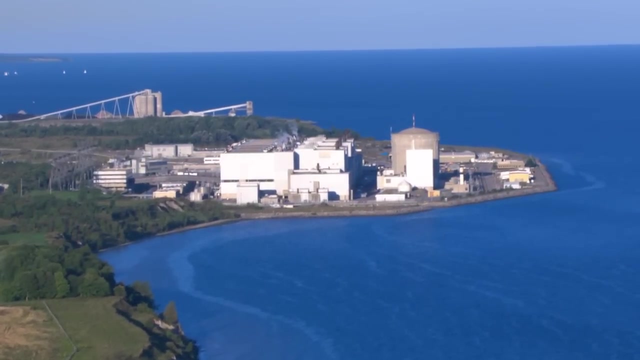 made of reinforced concrete. The fourth layer of containment is the building that houses and protects the reactor. The walls of the reactor building are made of at least one meter of reinforced concrete. The reactor building is surrounded by a one kilometer exclusion or buffer zone.